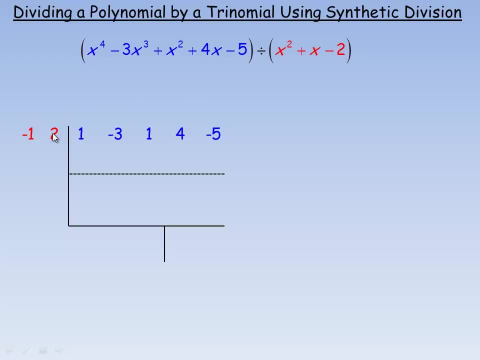 And that actually is the same for the constant at the end as when you're using synthetic division to divide by a binomial. Now the next thing you do is very similar to what you do in the normal synthetic division- is you bring this leading one all the way down here. 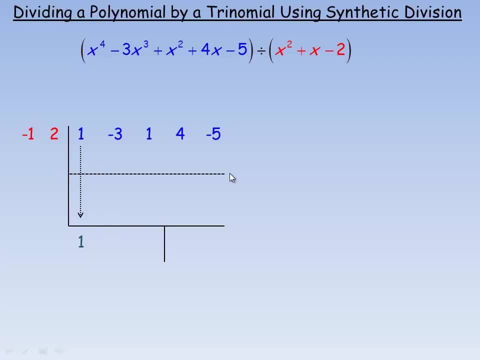 But because we're dividing by a trinomial and we have this extra row here, you also take this negative 3 and put it down here. Now you leave a space because there's going to be numbers below that. That's in the top of the two rows down here. 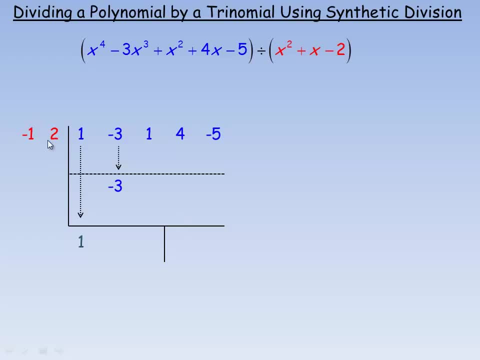 And what you do- and this next procedure is the same all the way through now- is you take this negative 1 and you multiply it by that 1.. And every time you multiply by the negative 1, here those numbers go in this row. 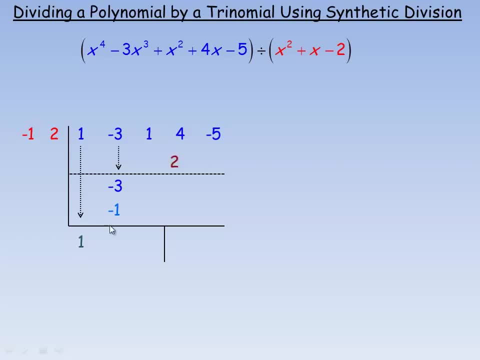 And so you also multiply the 2 by the 1.. And you always put those numbers in this row. So you put that 2, 2 times 1 is 2, right here, And the same as normal synthetic division. you add: 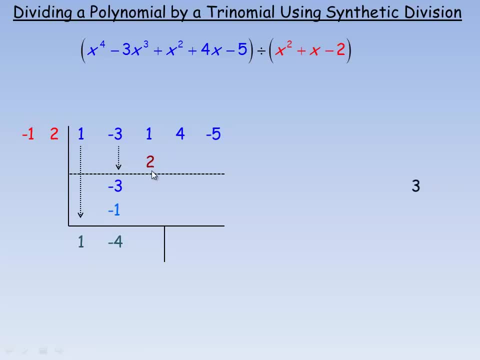 So negative 3 and negative 1 add to negative 4.. 1 and 2 add to 3.. Now we once again multiply negative 1 by negative 4, and of course that's positive 4.. So we put that here. 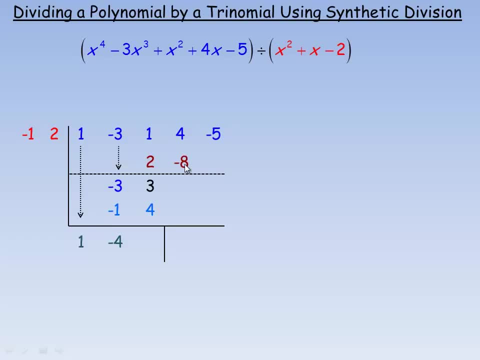 2 times negative 4 is negative 8, so that will go up here And we add again 3 and 4, add to 7.. 4 and negative 8, add to 2.. Negative, 4.. And so one last time: negative 1 times 7 would be negative 7 here. 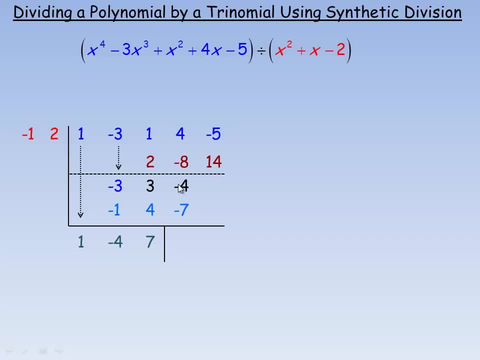 And 2 times 7 is 14, so we put that number up here. Negative 4 and negative 7 add to negative 11.. Negative 5 and 14 add to 9. And actually that 9 gets carried down here to go in the end. 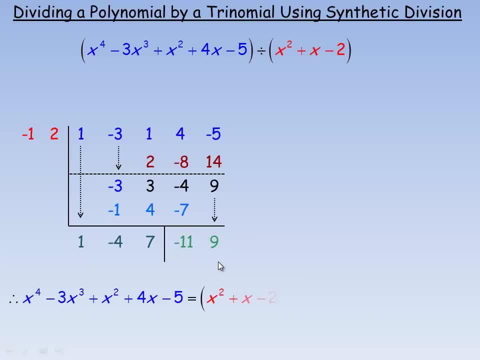 That's part of the remainder. So we divided this polynomial by x squared plus x minus 2.. And so the answer is: and the 1, negative 4, 7 means x squared minus 4x plus 7.. And the remainder is a negative 11x plus 9.. 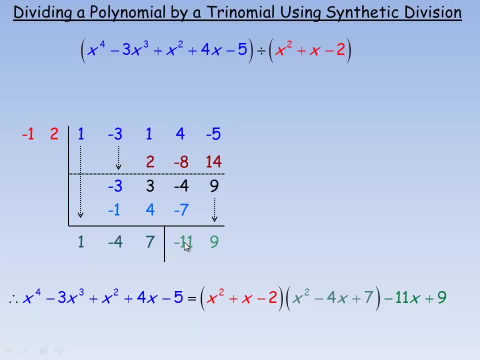 If you remember the way synthetic division goes: constant at the end, first power of x, second power of x, etc. So constant at the end, first power of x. that's why this is negative 4x to the first. This would be x squared. there's another one would be x cubed. 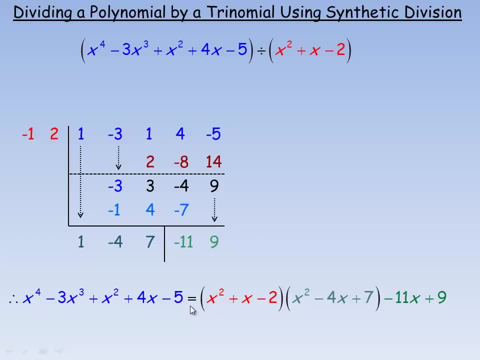 So one way to write out the division statement is because the polynomial we started with the quartic x to the fourth, minus 3x, cubed, plus x squared, plus 4x minus 5, would equal the product of: and it's basically this times this plus the remainder. 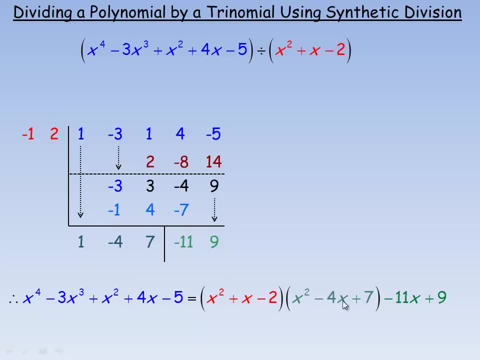 So the x squared plus x minus 2 times the x squared minus 4x plus 7, and the remainder is negative 11x plus 9.. Now if we take a look and compare this to the long division, you see a lot of similarities in the numbers. 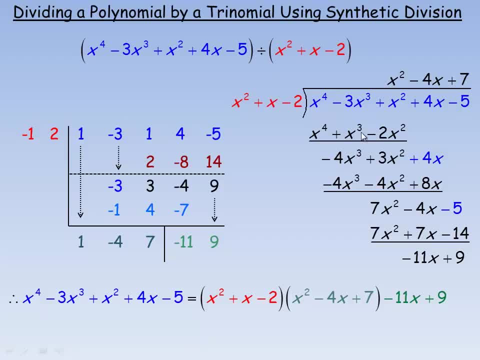 And the reason some of these signs are opposites. remember, in long division you subtract successive rows, in synthetic division you add, And if you remember, in long division, the coefficients 1x squared minus 4x plus 7, are actually these coefficients, right here? 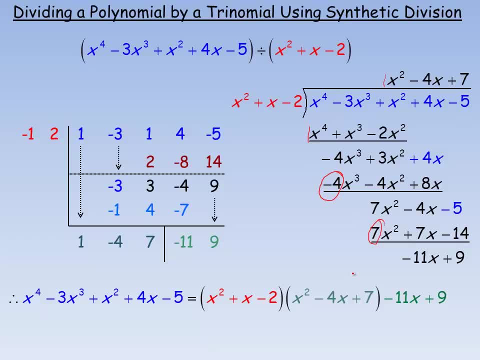 1, negative, 4, and 7.. And we find those, of course, right here: 1, negative, 4,, 7.. Now the coefficients in the rows, which are the 1,, the 1, and the negative 2 here: 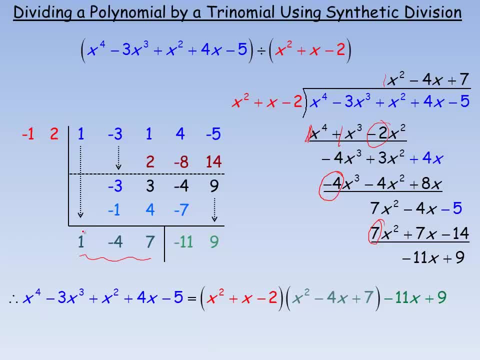 are. and now the first number is always the right sign, but the second number is always the opposite. So I said 1, 1, negative 2.. So these are the numbers actually right here: 1,. if I start the equation, 1, 1, negative 2.. 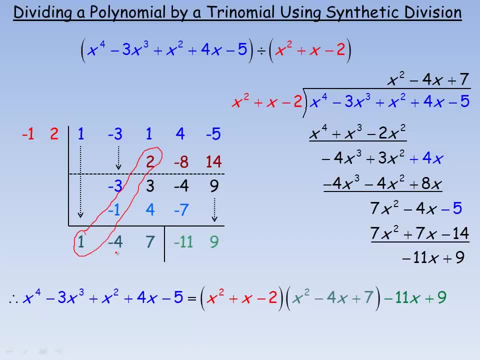 at the bottom left side, there 1,. now it goes negative 2, 2,. the second two numbers are always the opposite side and that's the difference between the adding and subtracting. If you look at the coefficients here, negative 4, negative 4, and 8,, that's these coefficients right here. 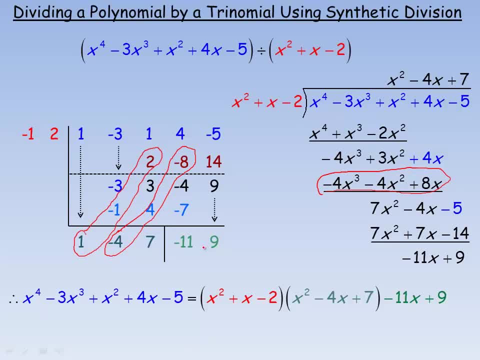 First number at the bottom is the same sign as in the long division. the second two numbers are opposites and the same, with the 7, 7, negative 14, 7 is correct or sorry, the same, and the second two are the opposite sign, and that's just the way that synthetic division works. 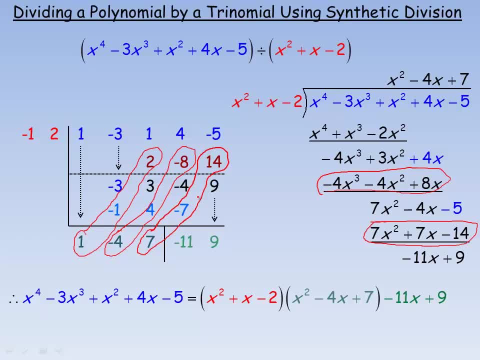 So that's the comparison between the synthetic and long division. but that's how synthetic division works when you're dividing by a trinomial.